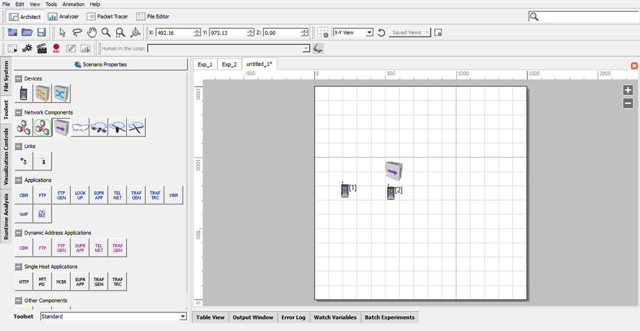 local area network which has been connected by using an hub like this. Okay, then go to the link section, connect interconnect. okay, this device, you can take more than two, It's not a problem. just for not to reduce the time or in order to make it simple, I'm 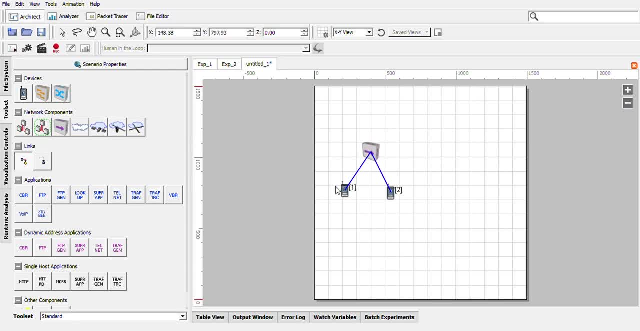 going with two, it is not a problem. just for not to reduce the time or in order to make it simple, I'm going with two simple local area network. okay, there you people. i think you people are familiar with this. okay, now i will go with an wireless network. can you see a cloud image like here? okay, click on the cloud. 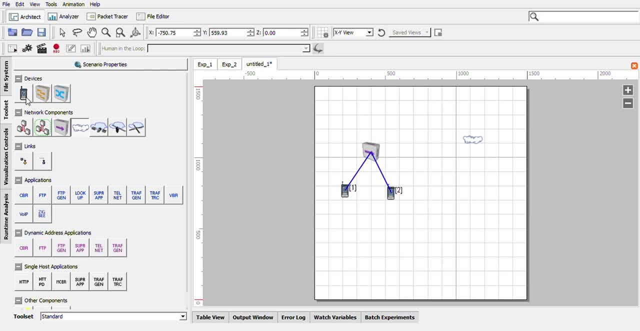 image and drop it here, okay. and if you want to connect uh nodes in the wireless network, okay, drop, okay, drop, like this. okay, either i can, i can take one more, also, no problem. and if you want to interconnect uh these nodes to the wireless network, uh, there are many ways. 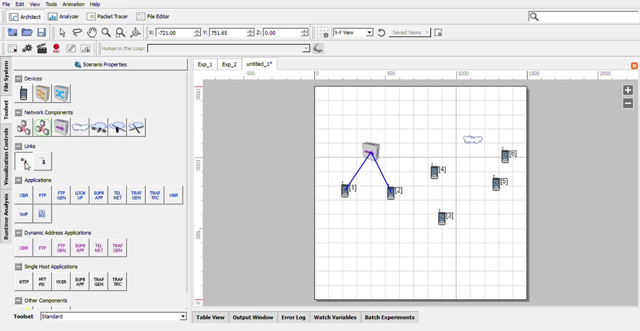 i will show you one simplest way. okay, again, go to the same point, to point link, which you have used to connect the nodes in case of local network. uh, as usual, start, click the most button, start from this one device and in it the other way. see, can you see? uh, now, this can you? i hope you can see. 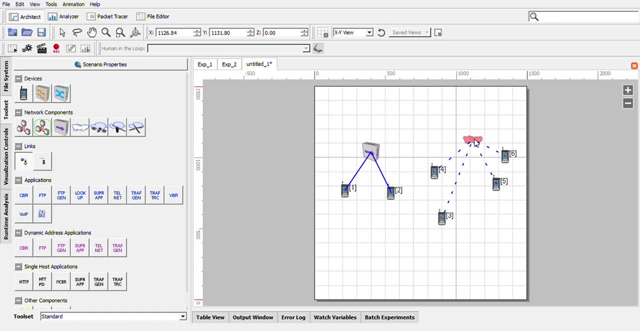 the difference visually, uh, this the dashed line indicator sits, and why a wireless uh connected. i mean, these nodes has been connected to this network through wireless manner or through air medium. okay, fine now. uh, as i said, i want to connect this network, wired network, to an wireless network. 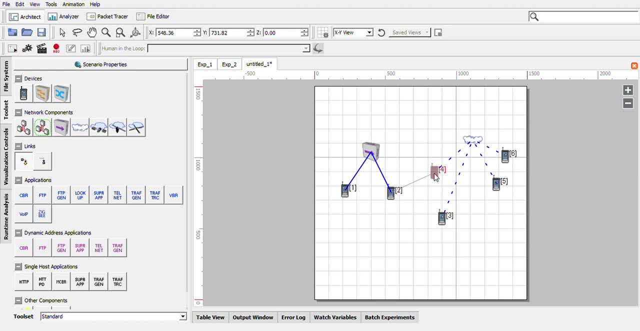 so obviously i, anyone nodes in this network, should be connected like this. so now, through this link, a wired network has been connected to the wireless network. and remember, if you click on the right- i mean right click on the cloud and go to the properties and go to the 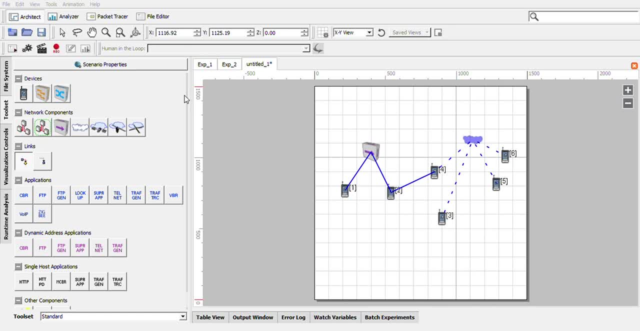 physical layer and make sure that uh the rate, by default, the radio type of that uh network, will be 802.11b, which is an ieee standard for wireless network. make sure that the radio type is this and even in the mac layer, make sure that the mac protocol that it is using is 802.11, which is 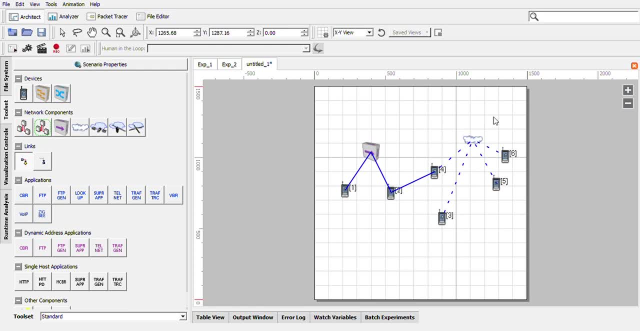 which stands for or which represent wi-fi network. so here this is an wi-fi network, this is a wide network and we have connected wide network with an wireless network. after this, take cbr applications run from node 2 to 3 means an application from wired network to an wireless network. then after this, as i said, you go to the. 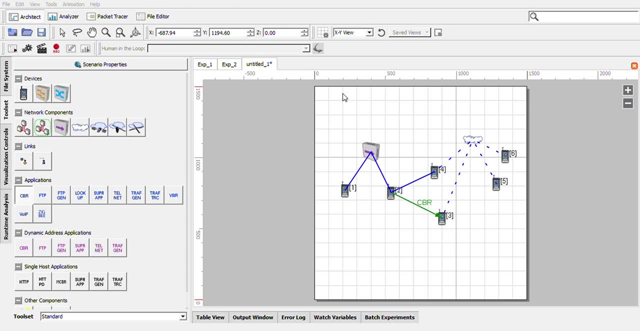 scenario properties and set the time to either 7000 or 8000, 6000, as i said in the previous videos, click apply. okay then right click on the application, go to the properties and let it send infinite number of packets and let it stop at 6000 seconds. okay then we created we. 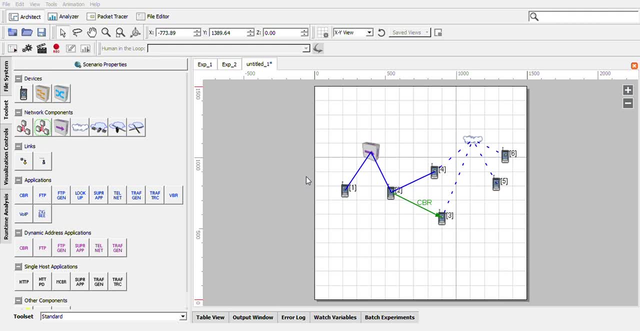 have suited this work to our works. so we are going to set the time to 5 second and then we will save our work, okay, and do the same as we did earlier: we will take the time and then we can save it. so it will save this work. we will save our work as experiment number three. 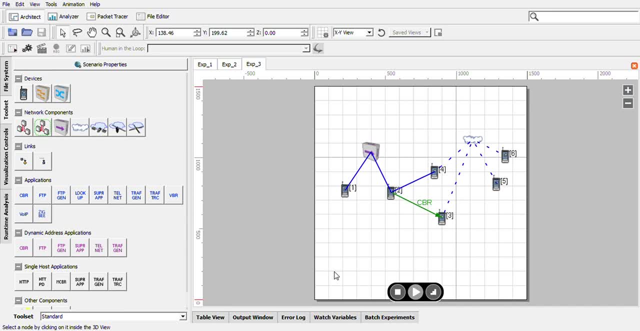 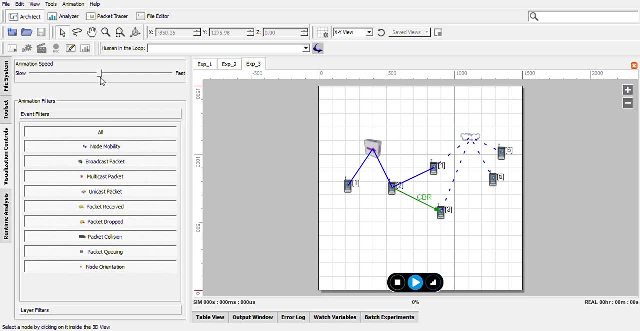 okay, then save. okay, now it will take time, few seconds or a few minutes, in order to get ready for simulation. okay, yeah, now it is ready. okay, then click on run so you can see a difference. okay, still, i think, if you go still to the again, if i click on run, 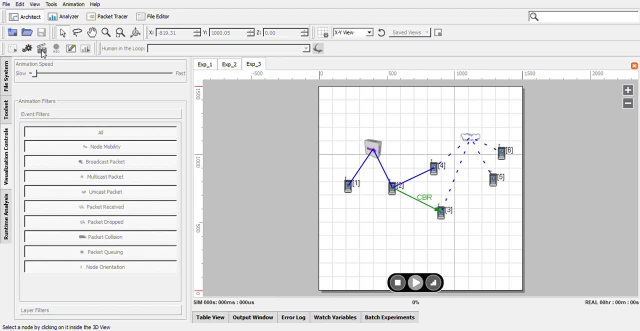 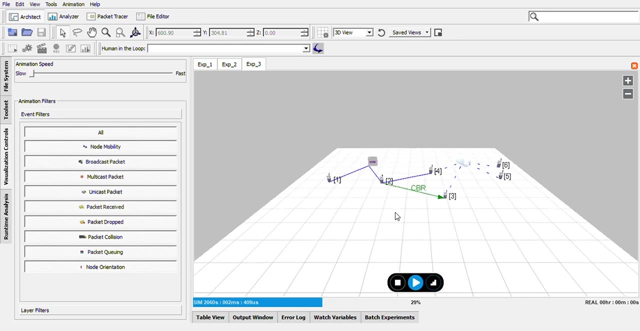 yeah, just for in order to make sure that you will find a sufficient difference between wide and wireless. just, i am going back. it is not again a rule. okay, click on next. okay, stop. okay, can you see the ranges? okay, i think you can better view this in 3d view. zoom it and now play. 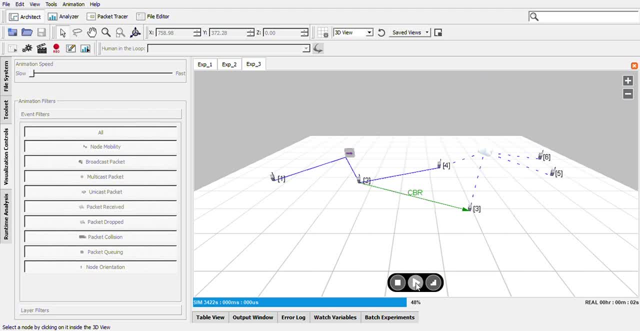 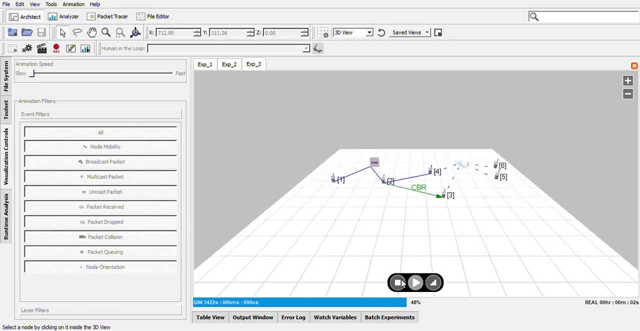 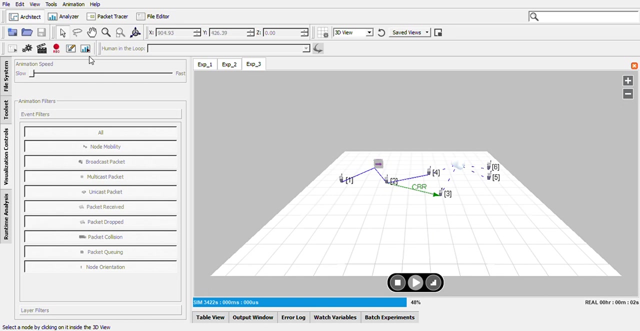 this see. okay, can you? did you observe? okay, i think, as i said, i am running in the server. it is taking time in order to okay, no problem, okay, i will continue. let it take time. okay, now let us see. uh, i hope we already have executed once. 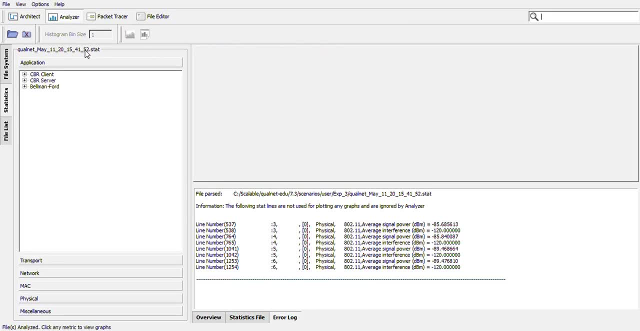 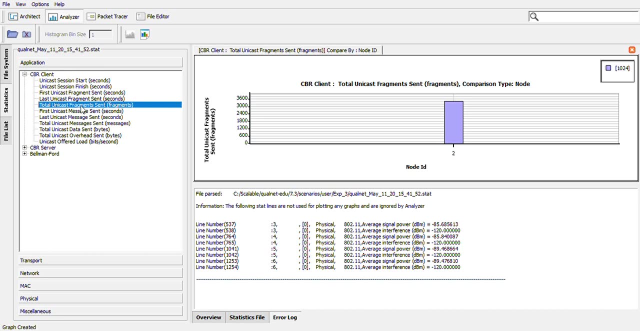 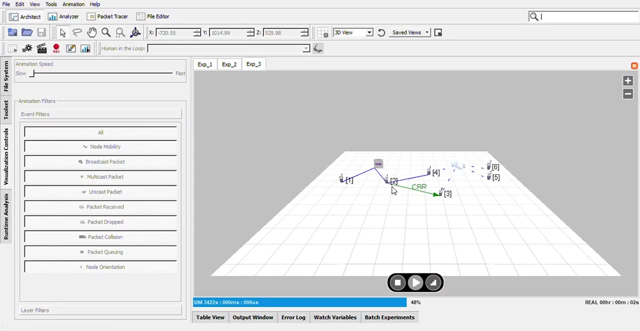 okay, go to the analysis part. okay that it has been updated. okay, make sure that both client and server are present here. okay, total unicast fragments sent by the sender: node two in this case receive total unicast fragments received: three, i think. two is the sender here. yeah, two is a sender here. three is a receiver here. okay, so this is what, again you. 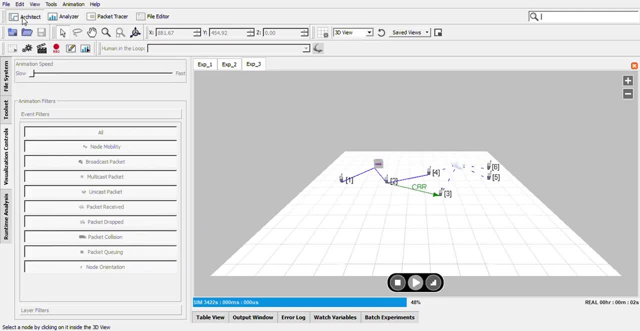 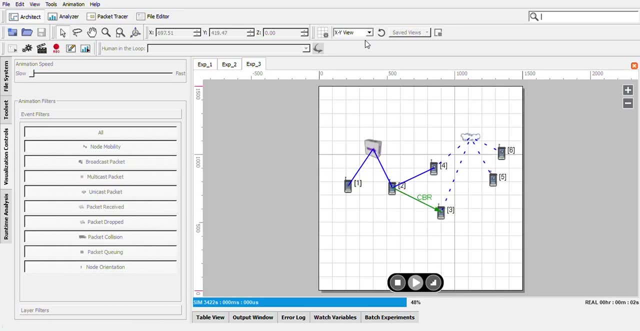 have to do is you have to check how many packets the client has and how many packets that the server has received. this is what you have to do. okay, this completes experiment number three. okay, and i, in the same video. i will continue with the experiment number four, where experiment number 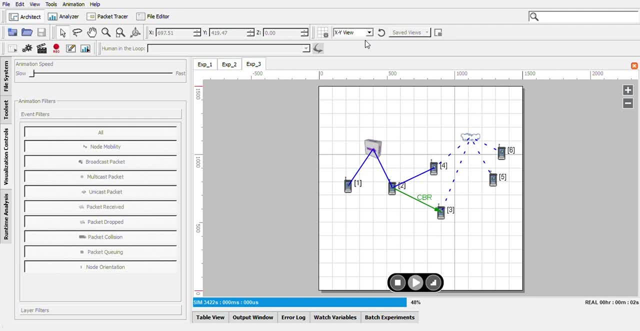 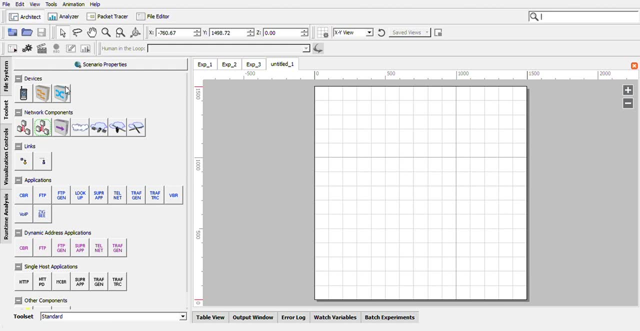 four, the objective is to you need to design or create a scenario for y max network. okay, it is very similar to experiment number three. i will show you how. it is very simple: go with a new. okay, then, as i said, uh, whenever you need an wireless network, the another way, the other. 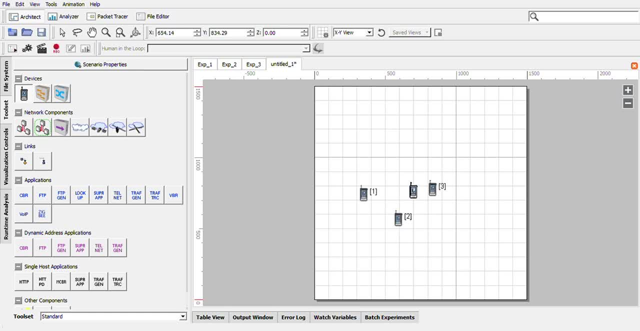 i will show you another way. so i will take only three nodes for simplicity. then i will take a cloud here. then go to the select icon, select it. or you can, or you can do like this: you can select if you want to delete. as i said, you can select or you can press delete key if you want to delete. 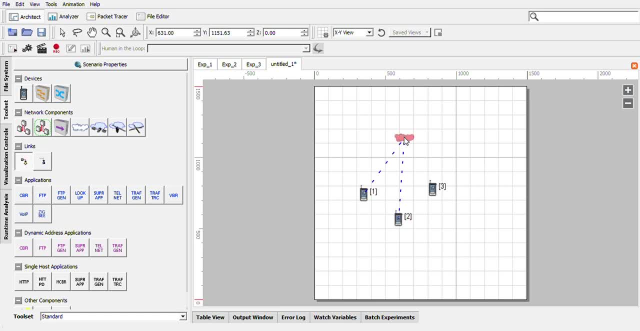 otherwise you can connect to this network like this. okay, and, as i said, this is this is by default. it is, it will be in wi-fi network, but our aim is we need to design a wimax network. wimax is a bigger than wi-fi network, so go to the properties- probably i mean cloud properties- go to physical layer and 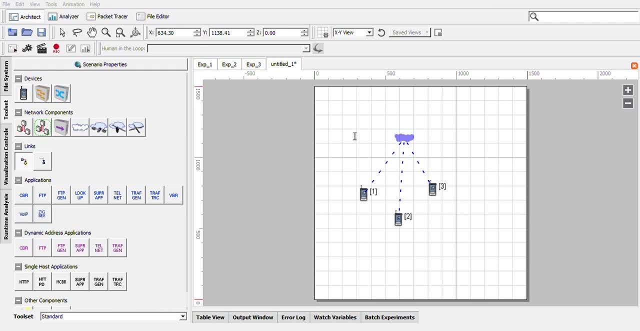 change this 802.11b to 16 radio, whereas 802.16 represent an ieee code or a standard for wimax network. change this to 802.16, even in mac layer. change to 802.16 and make sure that, by default, all the nodes are connected to the same network. so if you want to change this 802.11b to 16 and 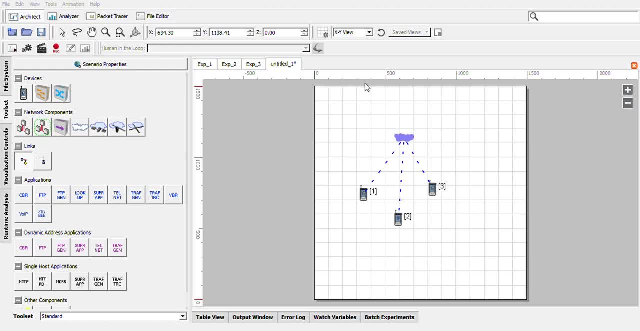 make sure that by default, all the nodes are connected to the same network. so if you want to, all station- i mean nodes in that network- become a subscriber station, okay, subscriber station means, uh, it's a station which is ready to subscribe to get a service from the base station. it, okay, see by. 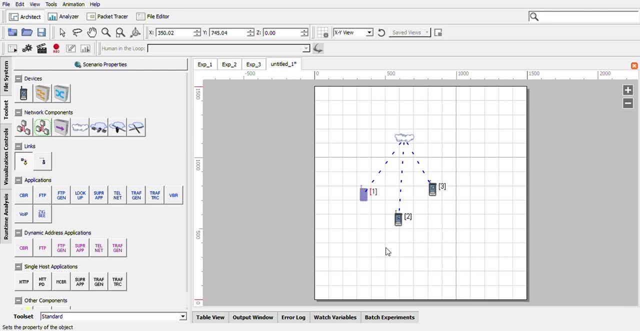 default, all these three are the subscriber station now, but one sender should be, always should be an. what base station? so i will teach you how to change this uh subscriber station to a base station. see right click or right click on that node properties and go to interfaces. go to interface. 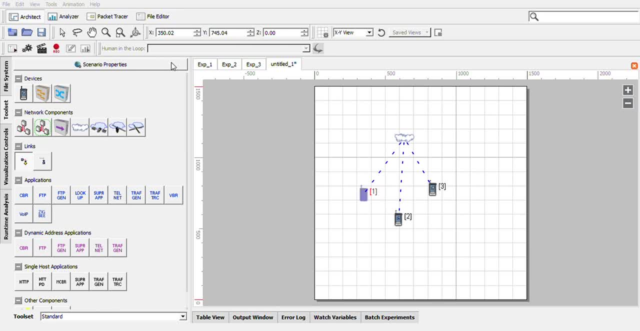 is: click on interface tab and click it here. go to the mac layer and see the station type is subscriber station. set it to base station. then don't worry about the. let it take default values. click apply. okay, now this acts like in base station. if you want to move, you can move, click. 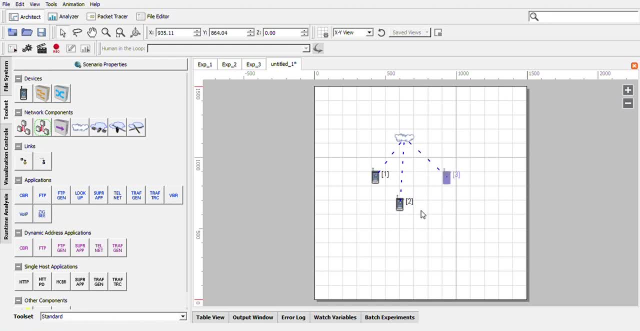 click on the select tool and you can move. like this, you can move. you can move like this: okay, like this, you can move, you can change. or you can move the position like this: okay, now these two are subscriber station, which is ready to to take a service from the base station. 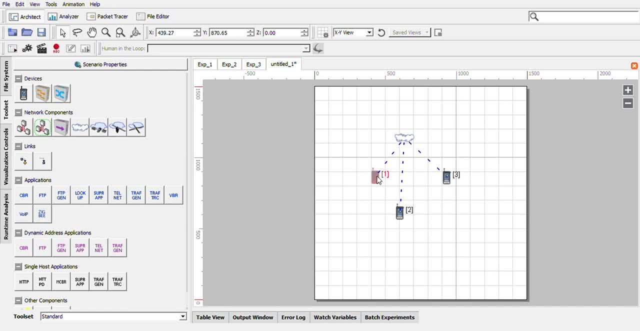 this base station number one, but there is no rule that you need to make one itself as a base station. you can make two or three as a base station. the other session subscriber station, but remember at least one node in the network should be a base station. then only it will work. 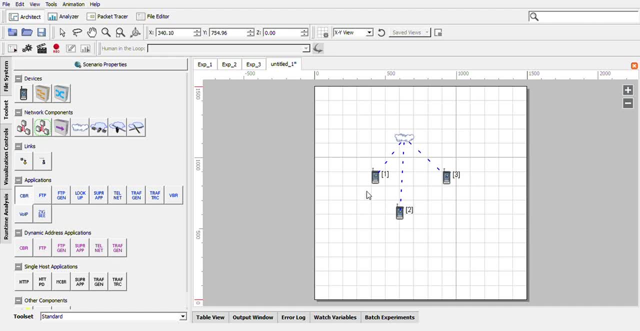 otherwise it will not work. okay, then i will run an application from one to two, then click on the properties, set it to as usual infinite number of packets and let it be 5000 seconds, and go to the scenario properties. as i said already, you can interchange the settings. no. 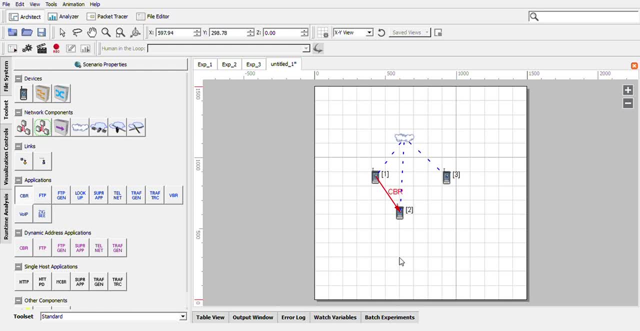 problem, but make sure that always this simulation scenario time should be bigger than the application time. okay then, after this, we we created, we configured, then go for running, then save this experiment as e experiment number four. okay then, as i said, since i'm running in the server, 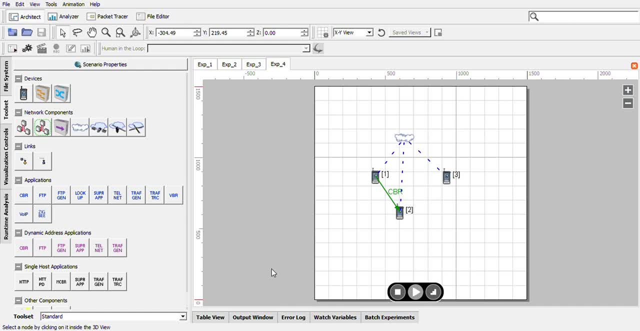 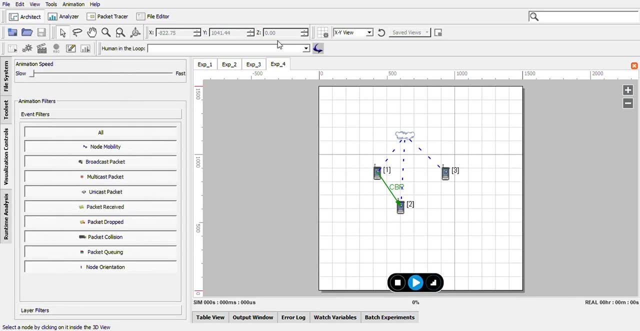 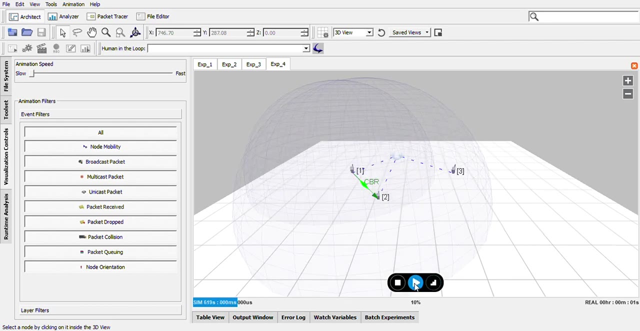 it will take a few seconds or minutes. let us wait. okay, it has not been. yeah, now it is ready. now make it to slow mode, change it to 3d. okay, now click on run. okay, now, see here. now see here they are interchanging and they are in range. so this is the range of imax network, if this node was.